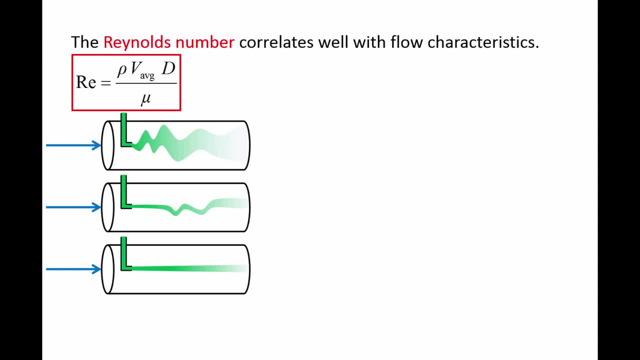 In the top pipe the dye always moves in an unpredictable manner and mixes with the surrounding fluid rapidly. The bottom pipe shows typical behavior of flows where the Reynolds number is less than 2300.. We call these type of flows laminar, and they are predictable and mix slowly. 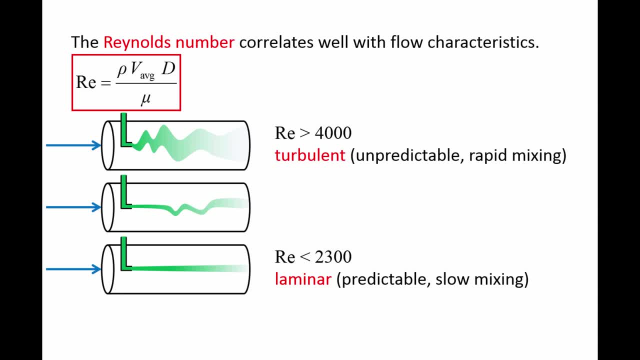 The top pipe shows typical behavior of flows where the Reynolds number is greater than 2300.. We call these type of flows turbulent, and they are unpredictable and mix rapidly. The middle pipe shows typical behavior of flows where the Reynolds number is between 2300 and 4000. 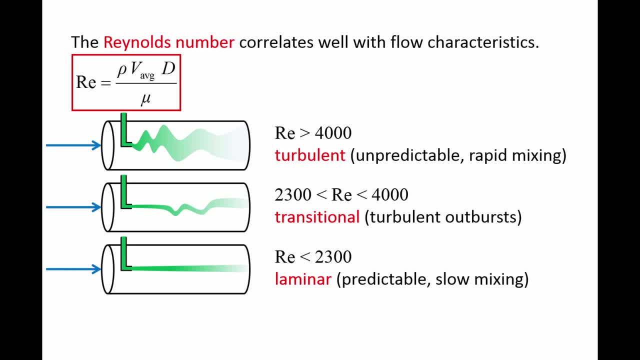 We call these type of flows transitional, and they have characteristics of both laminar and turbulent flows. It should be noted that 2300 and 4000 are only approximate cutoff values for laminar, transitional and turbulent behavior in pipes, For example. 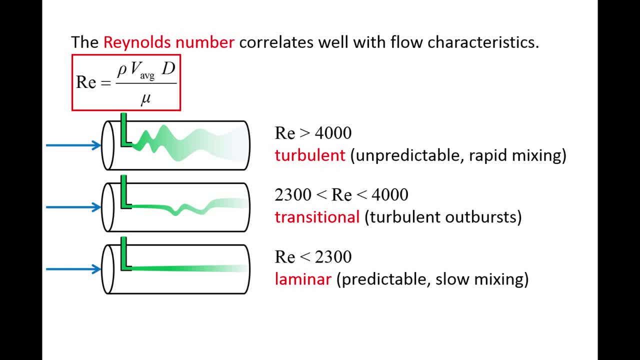 If great care is taken to not disturb the flow, it is possible to delay the onset of turbulence to Reynolds numbers that are much greater than 4000. However, under typical everyday conditions, the values of 2300 and 4000 are reasonable cutoff values. 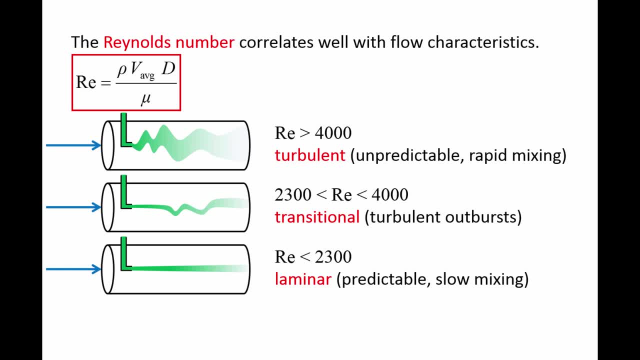 Notice that thus far we have not specified the flow speed, pipe diameter or type of fluid in the pipe. The Reynolds number cutoff values for laminar, transitional and turbulent flows are valid for any combination of flow speed, pipe diameter, density and viscosity. 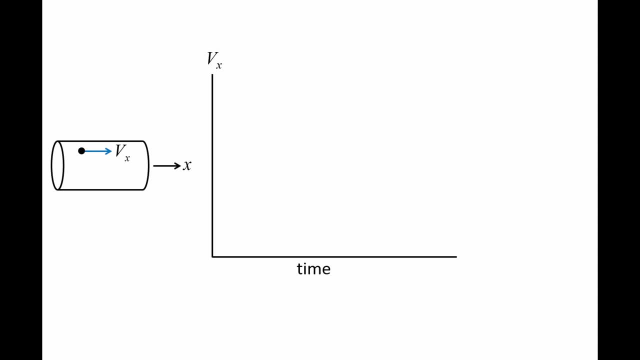 We can visualize the different flow regimes another way by examining the axial velocity component Vx at a single location in the pipe as a function of time. For laminar flows, the axial velocity component is constant in time. For turbulent flows, the axial velocity component varies unpredictably. 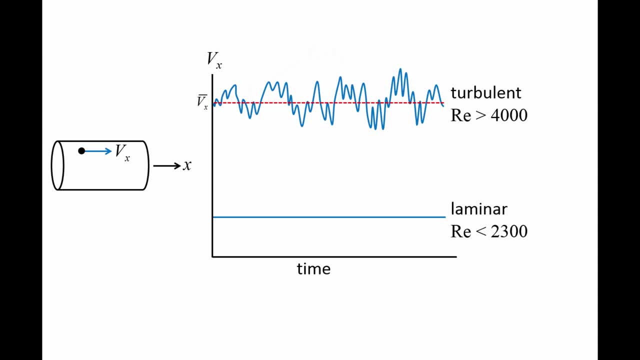 about a mean value, Vx bar. The axial velocity is expressed as the sum of Vx bar, which does not change in time, plus Vx prime, which is the deviation of the speed from the mean value. It is Vx prime which varies unpredictably in time. 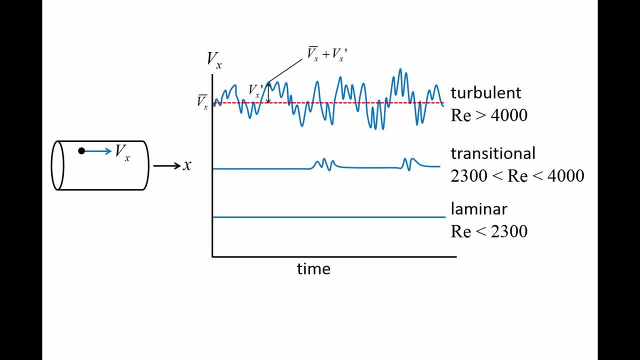 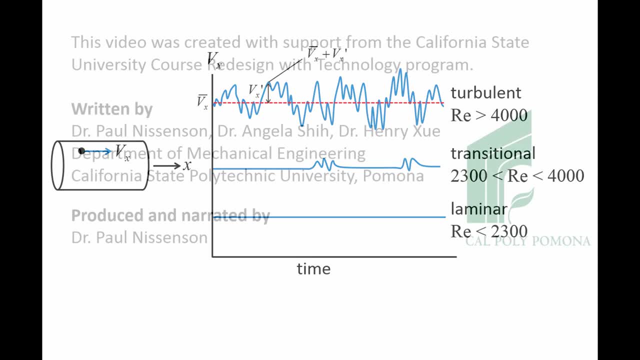 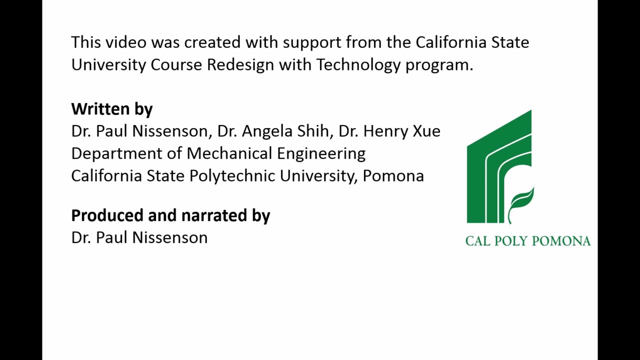 For transitional flows. the axial velocity component will appear constant at certain times and will vary unpredictably at other times. The axial velocity component also. it is Vx bar. There is a learning curve for y-axis flow in a particular Chernov token.